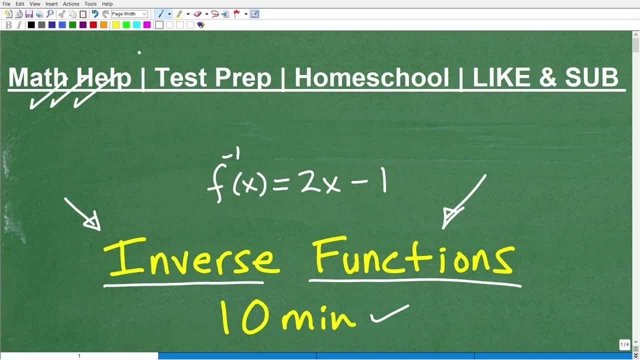 level and you need assistance in mathematics. I'm going to leave a link to my math help program in the description of this video. By the way, if you happen to be preparing for a test like the GED, SAT, ACT, maybe a teacher certification exam, anything with a math section, I can help you out. 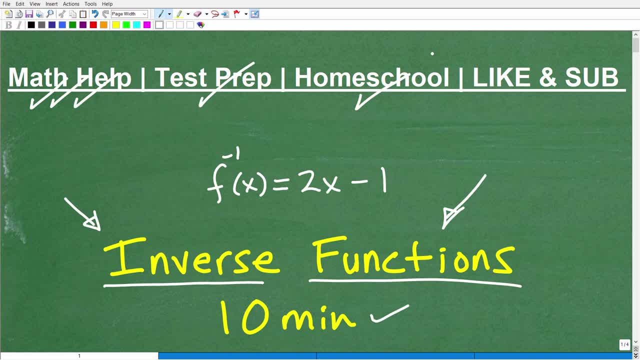 I also offer full homeschool math courses, And if this video helps you out, don't forget to like and subscribe, because that definitely helps me out. Okay, so let's go ahead and get started. Get into inverse functions. So I'm going to assume that you know something already about 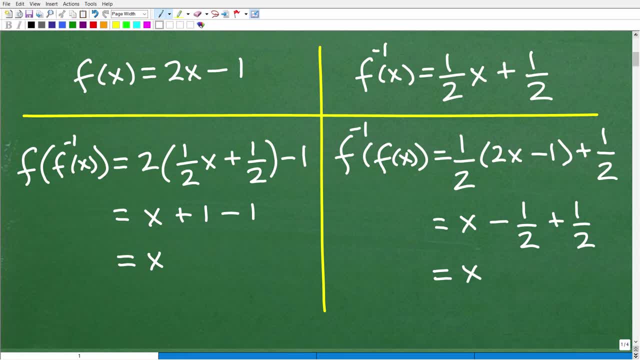 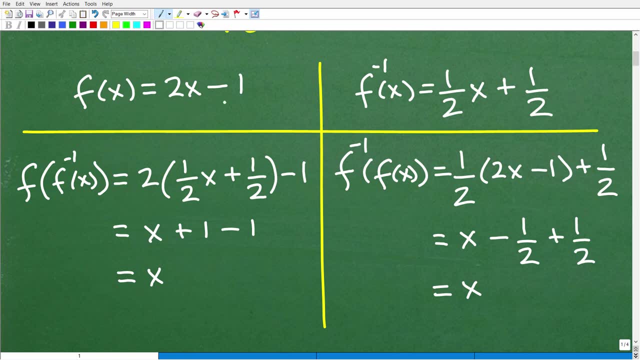 functions. Okay, And we're going to start off by just looking at the characteristics of how a function and its inverse, kind of like, behave. So here is a function And this function. right here, this little notation, this little negative one right there is, stating that this is the inverse. 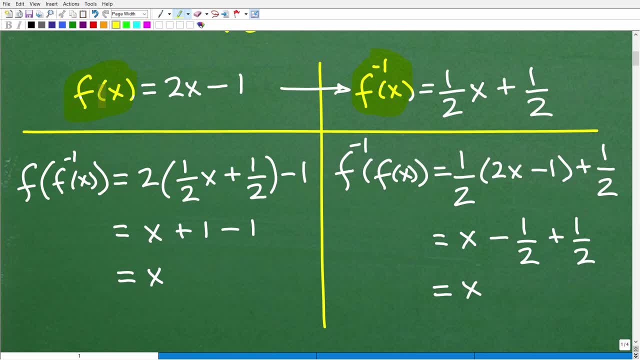 function of this function. So this is f of x. this is the inverse function of that function there. Now, here's the deal. This, if we just thought of this as a function, this function over here is the inverse of this function. Okay, so a function and its inverse is the same thing as the inverse function having 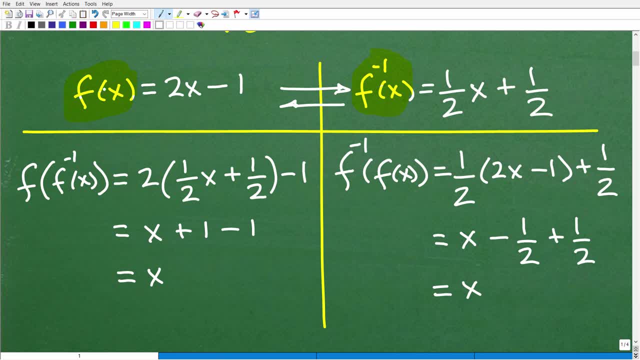 its function over here. So hopefully that's not too confusing. But here is how you know that you have an act, that you actually have an inverse function. I'm going to get into how to find the inverse function. all that good stuff. Just let's just kind of first get a general idea. 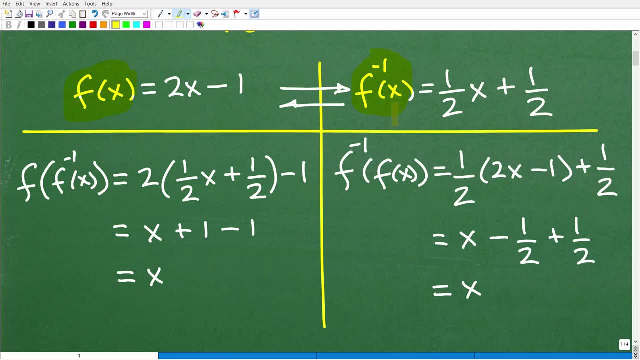 of what a function and a function are. Okay, so let's take a look at what a function and an inverse function do. Now, if you take a composite function, let's take this f of x function here And let's plug in the inverse function right there. 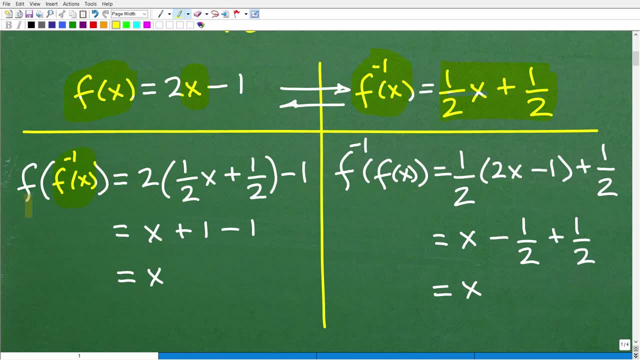 Okay, so in other words, we're going to plug all this stuff in there. That's, that's what this notation is saying. So if you don't understand function operations, especially composite functions, which is kind of a confusing thing for a lot of algebra students, Let me give you a 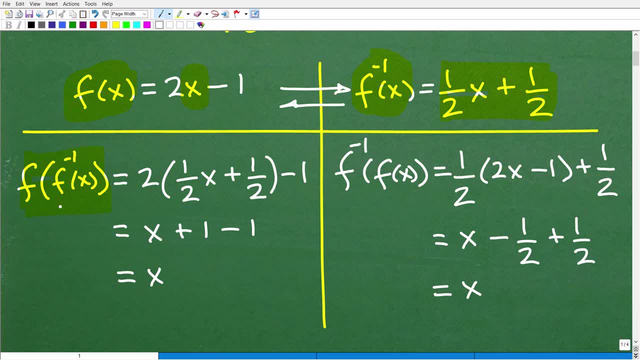 couple suggestions. One: I got tons of videos on this stuff on my YouTube channel And then also you may find a lot of videos on my YouTube channel, And then also you may find a lot of videos on my YouTube channel. So if you want to check out, like my full algebra course. but let's go ahead and plug in the inverse. 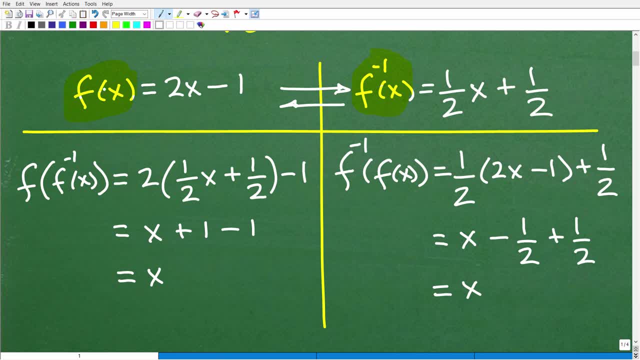 its function over here. So hopefully that's not too confusing. But here is how you know that you have an act, that you actually have an inverse function. I'm going to get into how to find the inverse function. all that good stuff. Just let's just kind of first get a general idea. 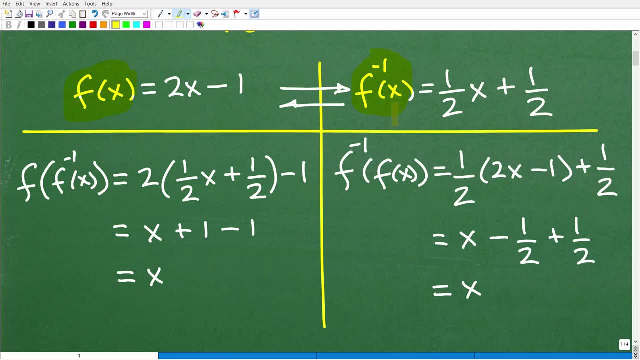 of what a function and a function are. Okay, so let's take a look at what a function and an inverse function do. Now, if you take a composite function, let's take this f of x function here And let's plug in the inverse function right there. 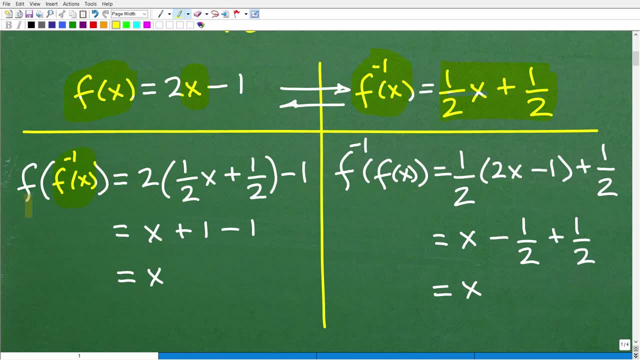 Okay, so in other words, we're going to plug all this stuff in there. That's, that's what this notation is saying. So if you don't understand function operations, especially composite functions, which is kind of a confusing thing for a lot of algebra students, Let me give you a 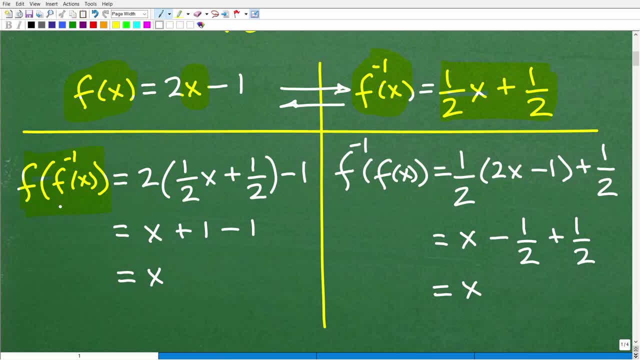 couple suggestions. One: I got tons of videos on this stuff on my YouTube channel And then also you may find a lot of videos on my YouTube channel And then also you may find a lot of videos on my YouTube channel You might even want to check out, like my full algebra course. But let's go ahead and plug in the 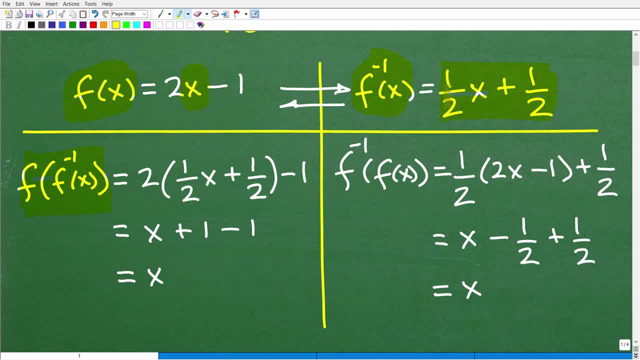 inverse function into this function. So I'm going to replace this x with the inverse function. This is finding the composite function right, So we're plugging in the inverse into this function. So you can see here this setup. Now, when I simplify this, I'm going to get two times one half x plus. 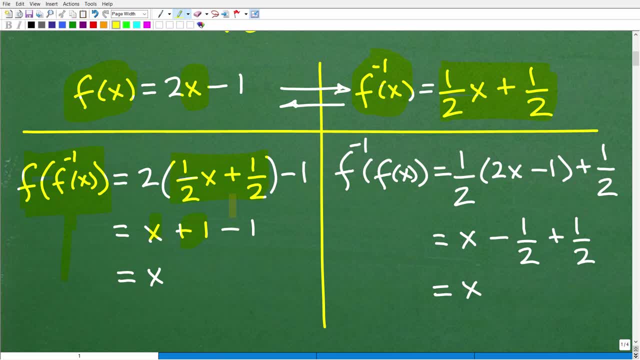 one half. you're going to get x plus one here, minus one, Okay, so hopefully you understand that, But really this simplifies down to just x. okay, now let's go ahead and plug the function into the inverse function. let's see what happens. so we're going to plug in this function right here into this inverse function. 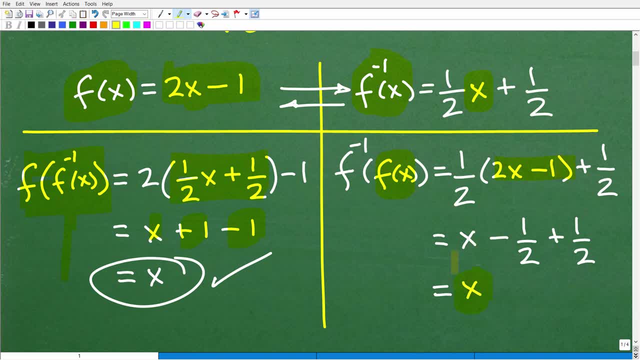 and when i do that, you can kind of just see all this math here we also end up with x, okay, so basically a function and an inverse kind of undo one another and you'll end up with x. this is basically the definition of a function inverse, that basically both composite functions here. 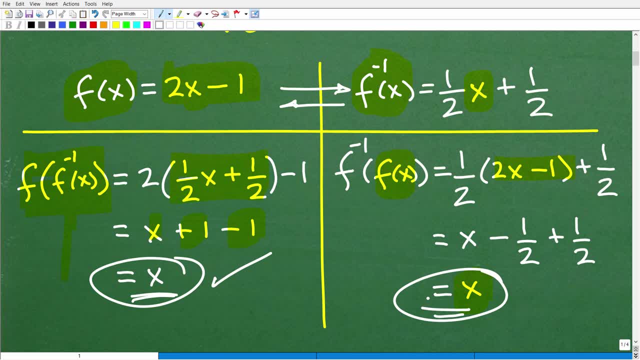 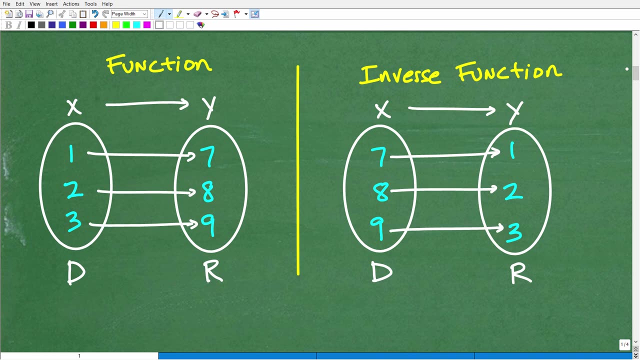 end up as equal. they end up equaling to x, okay. but you can kind of think of again: a function and its inverse is kind of undoing one another. all right, let's take a look at a function and the inverse function this way, okay. so hopefully you're familiar with a mapping diagram. 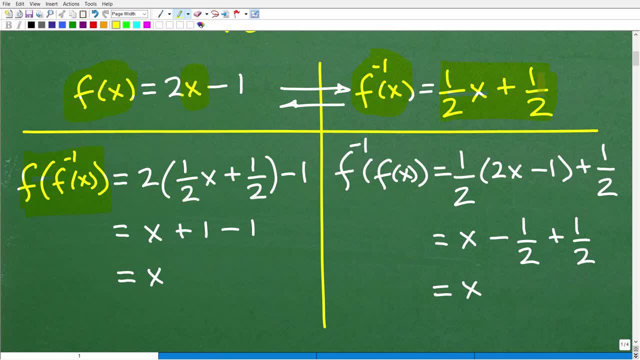 function into this function. So what? I'm going to replace this x with the inverse function. this is finding the composite function right, So we're plugging in the inverse into this function. So you can see here this setup. Now, when I simplify this, I'm going to get two times one half x plus one half. 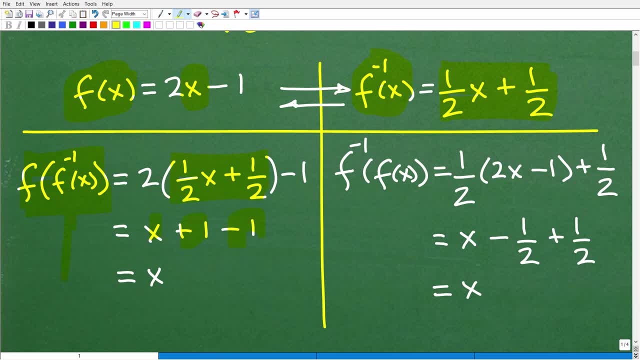 I'm going to get x plus one here minus one, Okay, so hopefully you understand that. But really this simplifies down to two times one half x plus one half, And then I'm going to get two times one half x plus, down to just x. Okay, Now let's go ahead and plug the function into the inverse function. Let's see. 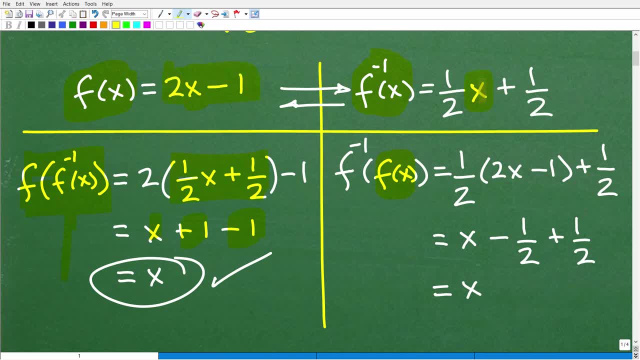 what happens. So we're going to plug in this function right here into this inverse function, And when I do that you can kind of just see all this math here We also end up with x. Okay, so basically a function and an inverse kind of undo one another and you'll end up with x. This is 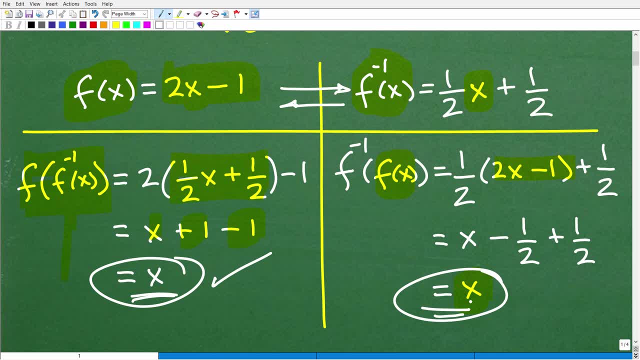 basically the definition of a function inverse, That basically both composite functions here end up as equal. they end up equaling to x, Okay. but you can kind of think of again: a function and its inverse is kind of undoing one another, All right. 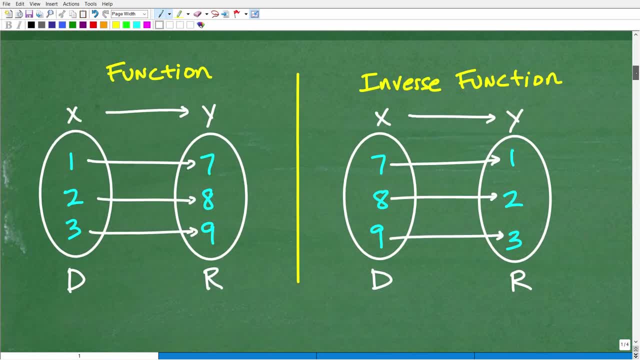 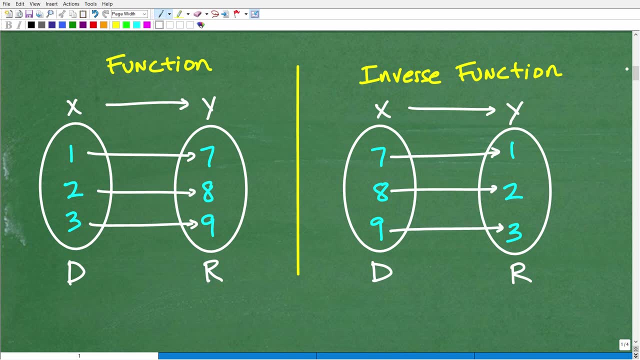 let's take a look at a function and the inverse function this way. Okay, so hopefully you're familiar with a mapping diagram. If you're not, you definitely need to be familiar with this. But let's focus on this here. This could be a 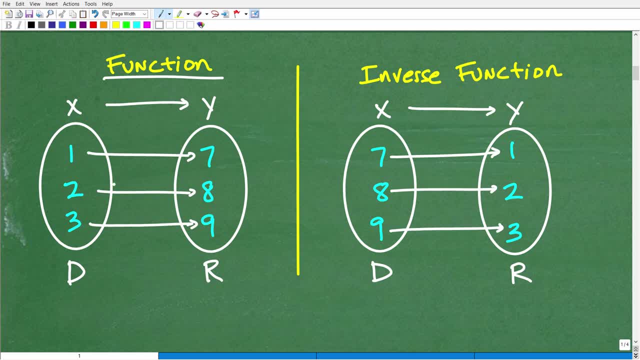 simple mapping diagram of a function. There's a lot of ways we can express functions And this right here is basically stating this function. here One is pointing to seven, So that represents the point one, seven. Two is pointing to eight. That's the point two, eight, And then three is pointing to 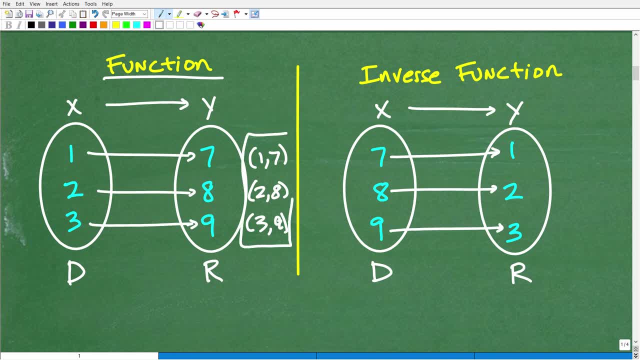 nine, That's the point three. nine. So this set of points collectively is a function, because when we map it out here we don't have any x trying to point to one and, oh, two or more y's. Okay, so that's the definition of a function: Every x. 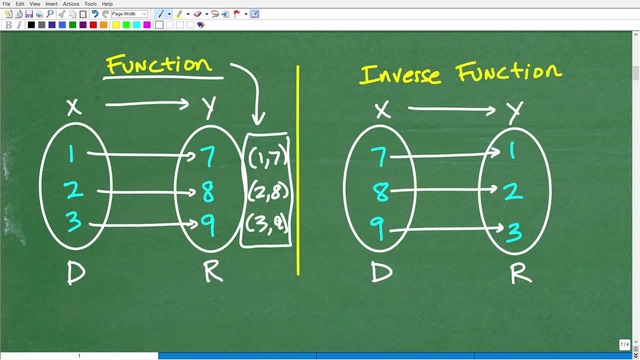 points to one and only one, y. So if you don't really understand the definition of a function, again, I have tons of videos on this. If you really want to master this stuff, check out any one of my algebra courses from pre-algebra: algebra one. algebra two: 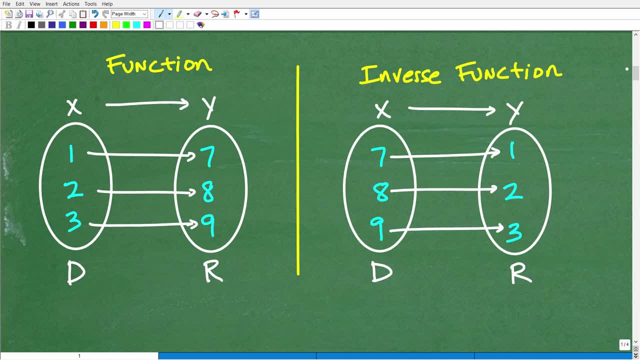 if you're not, you definitely need to be familiar with this, but let's focus on this here. this could be a simple mapping diagram of a function. there's a lot of ways we can express functions, and this right here is basically stating this function. here one is. 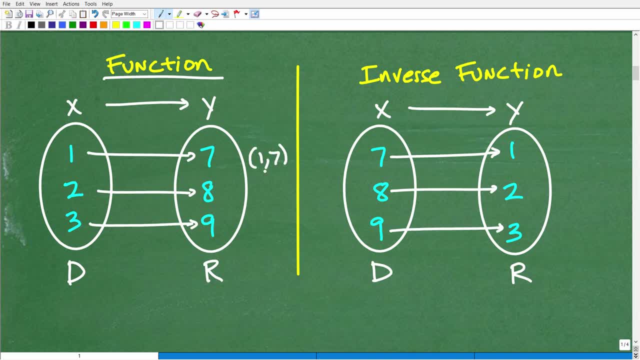 pointing to seven. so that represents the point one. seven, two is pointing to eight. that's the point two. eight and then three is pointing to nine. that's the point three. nine. so this set of points collectively is a function, because when we map it out here we don't have any x trying to point to. 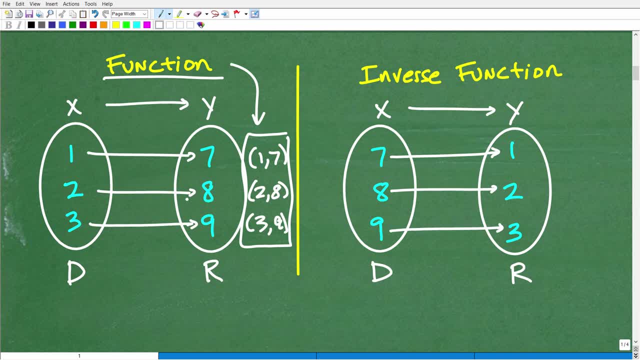 one and two or more y's okay. so that's the definition of a function. every x points to one and only one y. so if you don't really understand the definition of a function, again i have tons of videos on this. if you really want to master this stuff, check out any one of my. 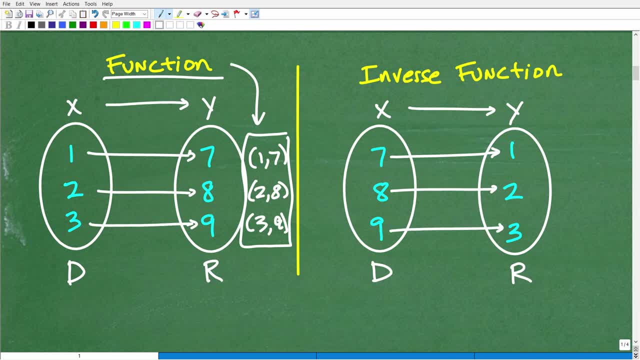 courses from pre-algebra, algebra one, algebra two, college algebra and then my most advanced stuff would be in pre-calculus. but anyways, let's take a go back to this function here. so the domain is the set of all of our input values and it's uh associated with the variable. 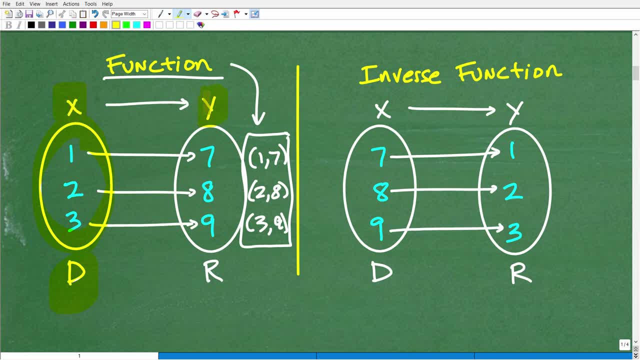 x, this is our uh- independent variable, and y is the dependent variable, and this right here, all these values, is our range. okay, so you should know this. this is the domain, this is the range of this function. now let's take a look at the inverse function. so this function here, let's take a look at its inverse. okay, so this would be the inverse function. 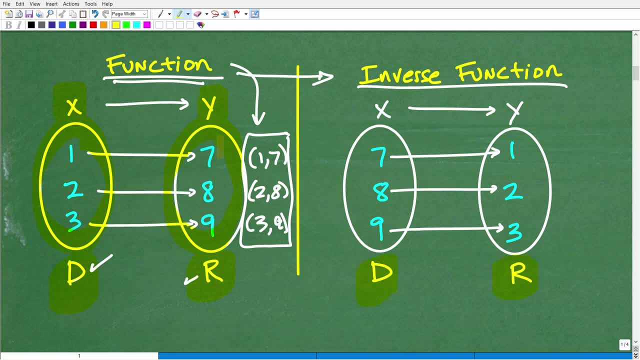 now let's look at the domain and range. notice here that the range of the function is now the domain of the inverse function and the domain of the function is now the range of the inverse function. okay, so, anyways, these are things that you need to know, all right, when you have a function. 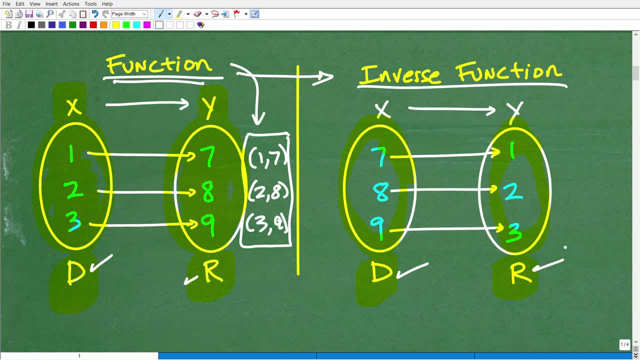 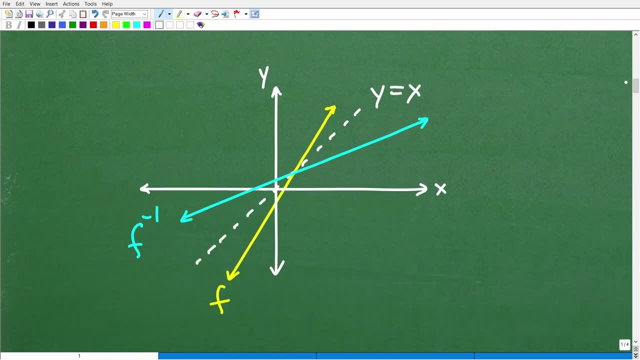 and it's inverse. the domain and range switch around. okay, so hopefully i can keep this lesson around 10 minutes. i'll probably go a little bit over, but it'll be worth your time, as you're going to learn a lot about inverse functions. okay, so let's talk. 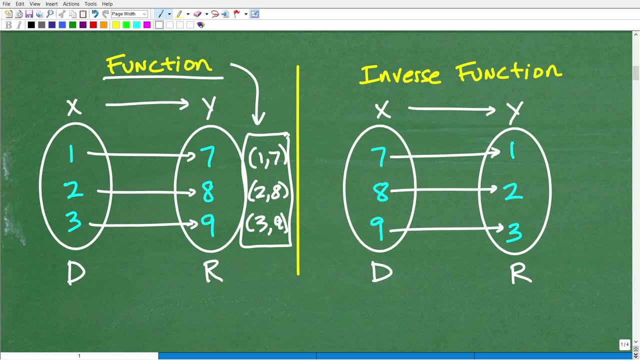 college algebra, and then my most advanced stuff would be in pre-calculus. But anyways, let's go back to this function here. So the domain is the set of all of our input values and it's associated with the variable x. This is our. 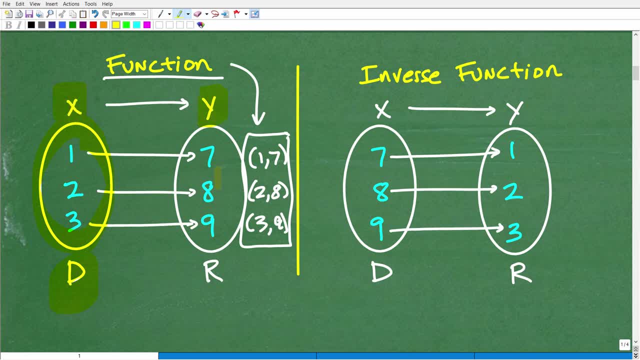 independent variable and y is the dependent variable. And this, right here, all these values, is our range. Okay, so you should know this. This is the domain, This is the range of this function. Now let's take a look at the inverse function. So this function. here let's take a look at its. 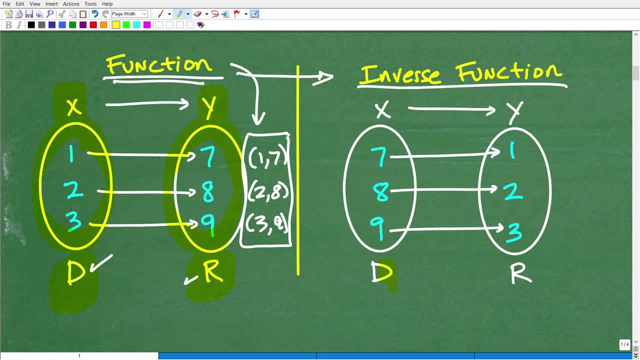 inverse. Okay, so this would be the inverse function. Now let's look at the domain and range. Notice here that the range of the function is now the domain of the inverse function And the domain of the function is now the range of the inverse function. Okay, so anyways. 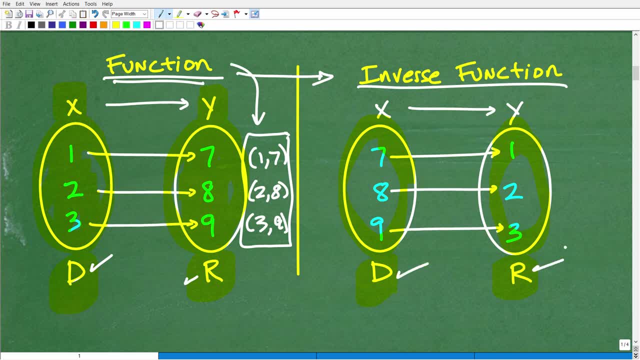 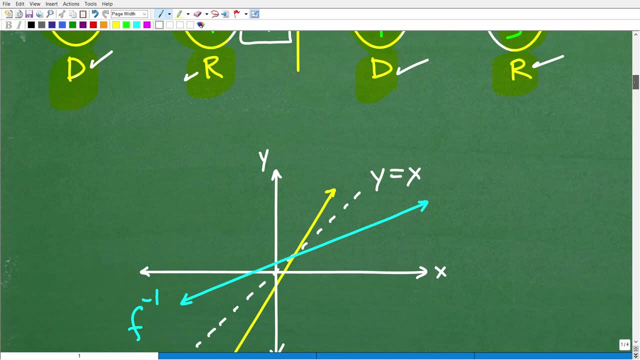 these are things that you need to know. All right, when you have a function and it's inverse, the domain and range switch around. Okay, so hopefully I can keep this lesson around 10 minutes. I'll probably go a little bit over, but it'll be worth your time, as you're going to learn. 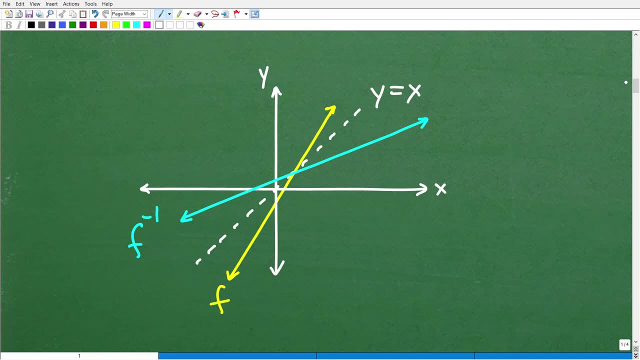 a little bit more about the inverse function. So let's get started. Let's get started. Let's get started. a lot about inverse functions, Okay, so let's talk about another: characteristics of functions and their inverse, And that is this: If you were to graph a function and its inverse, assuming that, 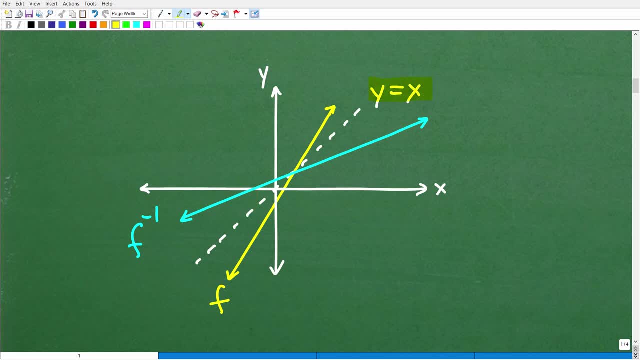 function has an inverse, and I'm going to get into that here in a second. the graphs would be symmetric along the y equals x line. So here is the y equals x line. If you don't know how to graph lines, well, you need to go back and review how to do that. But here is the y equals x line. 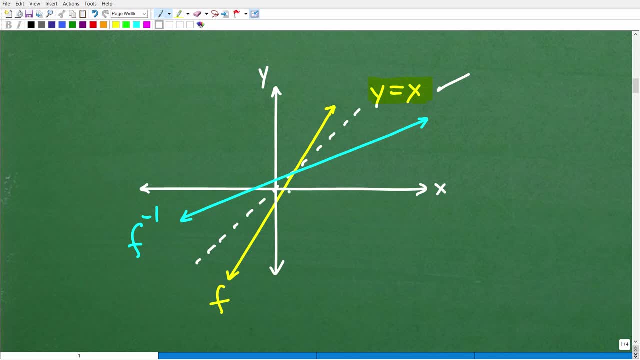 so let's suppose this yellow line represents the graph of a function, Okay, and its inverse would be this blue line: Okay. but if I was to graph the inverse and the function, they would be symmetric, ie, they would be, they would form a mirror image over this line. Okay, this will always. 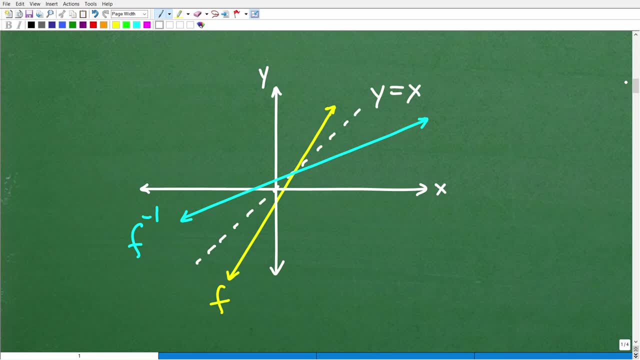 about another characteristics of functions and their inverse, and that is this: um, if you were to graph a function and its inverse- assuming that function has an inverse, and i'm going to get into that here in a second- the graphs would be symmetric along the y equals x line and 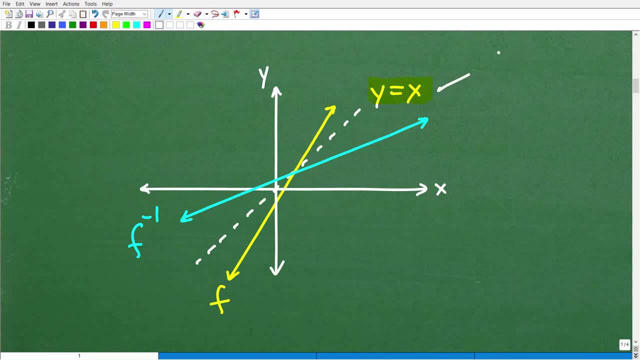 so here is the y equals x line. if you don't know how to graph lines, well, you need to go back and review how to do that. but here is the y equals x line. so let's suppose this yellow line represents the graph of a function, okay, and its inverse would be this blue line- okay. but if i was, 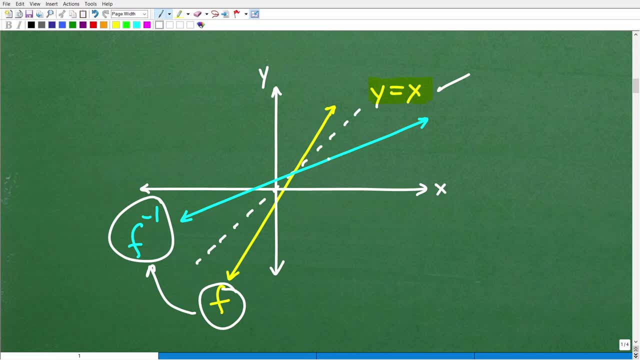 to graph the inverse and the function. they would be symmetric, ie, there would be. they would form a mirror image over this line. okay, this will always be the case, uh, between a function and inverse, right, when you graph them, uh, they will the graphs of the function and the inverse will. 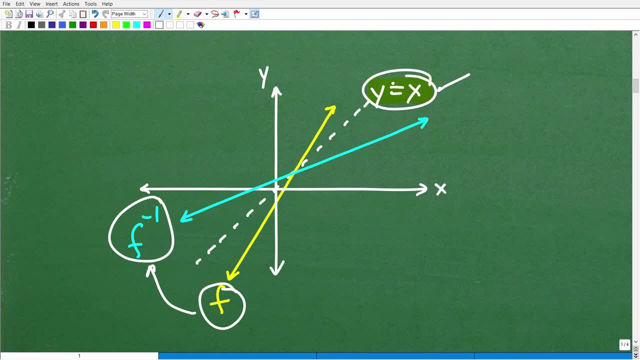 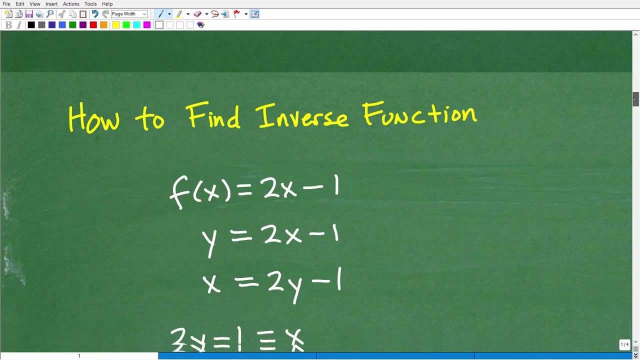 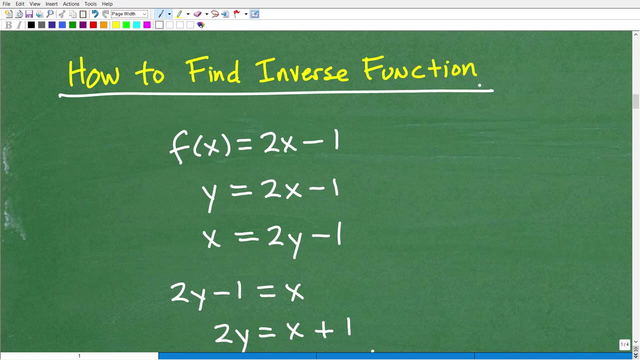 be symmetric again across this y equals x line. these are things that your teacher is going to expect you to know, okay? so let's move on and talk about how to find an inverse function. now i'm going to tell you right now. not all functions have inverses, so somebody might be saying, wow, what? 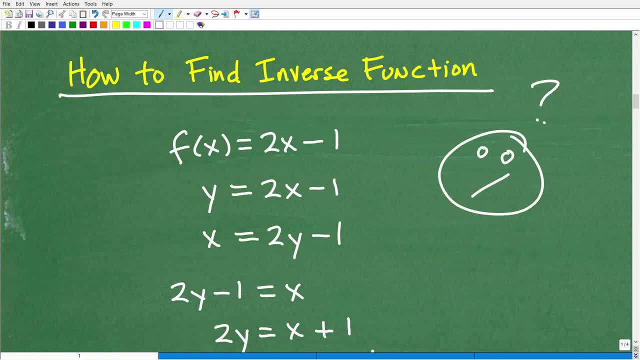 is this guy talking about? not all functions have inverses. well, how do you know? well, i'm going to tell you that here in a second. but let's go ahead and assume that a particular function that you're given does have an inverse. so how do you go about doing that? 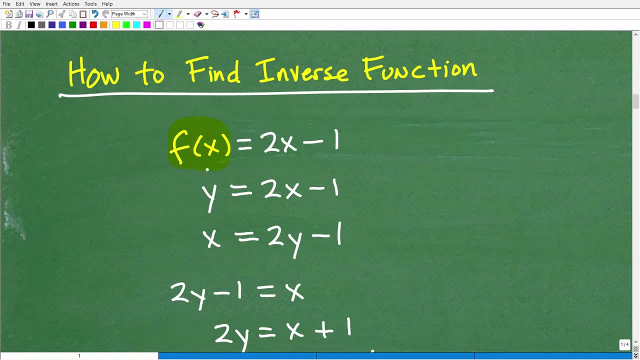 well, this is the steps you need to follow. all right, so the first thing you need to do is you need to understand when you have f of x, this function notation, f of x is always equal to y. okay, so i can replace this f of x with a y, and you need to do that because our first step 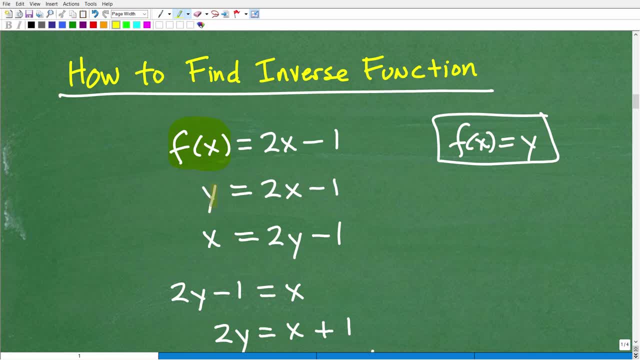 to find. the inverse function is the following: so here's your y, here's your x. what you're going to do is replace the x with the y and the y with the x. so, right here, i'm going to put a y, and then, right here, i'm going to put an x. so the first step is, after you write your function with a y, you're. 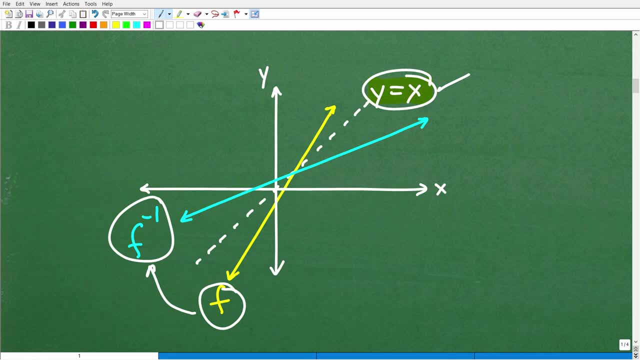 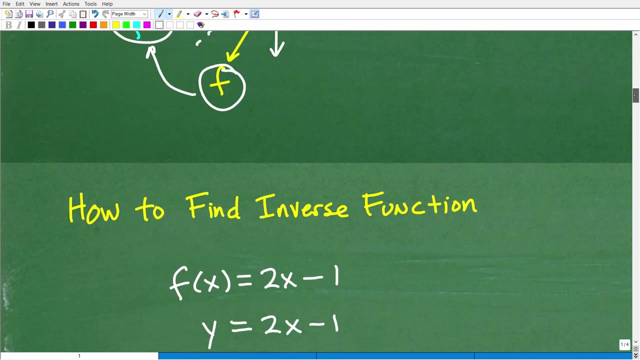 be the case between a function and its inverse. right When you graph them, they will. the graphs of the function and the inverse will be symmetric again across this y equals x line. These are things that your teacher is going to expect you to know, Okay, so let's move on and talk about. 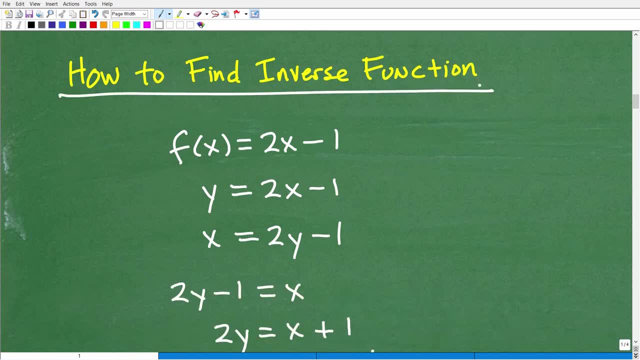 how to find an inverse function. Now I'm going to tell you right now: not all functions have inverses. So somebody might be saying: well, what is this guy talking about? Not all functions have inverses. Well, how do you know? Well, I'm going to tell you that here in a second, but let's go. 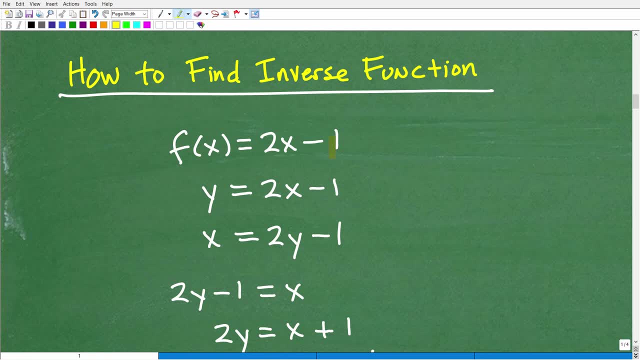 ahead and assume that a particular function that you're given does have inverses. So let's go ahead and assume that you have an inverse. So how do you go about doing that? Well, this is the steps you need to follow. All right, so the first thing you need to do is you need to understand when you have 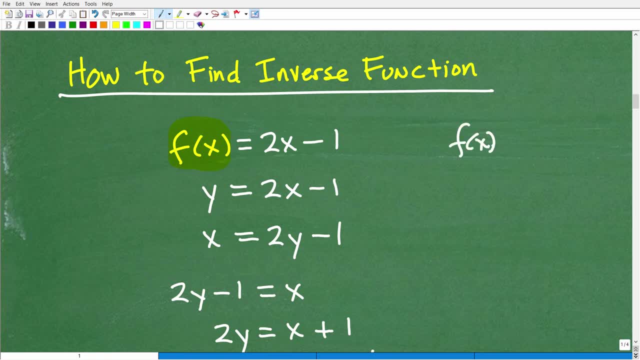 f of x. this function notation f of x is always equal to y. Okay, so I can replace this f of x with a y, and you need to do that because our first step to find the inverse function is the following: So here's your y, here's your x. What you're going to do is replace the x with. 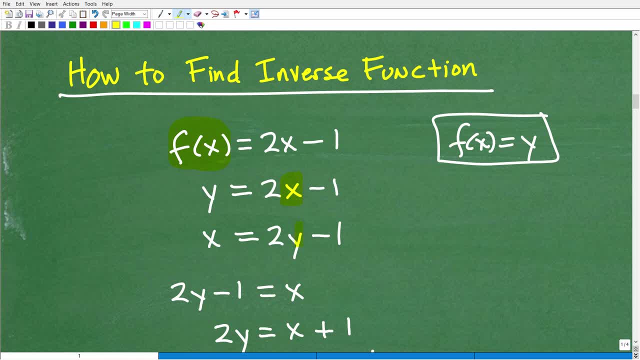 the y and the y with the x. So right here I'm going to put a y and then, right here, I'm going to put an x. So the first step is, after you write your function with a y, you're going to flip-flop. 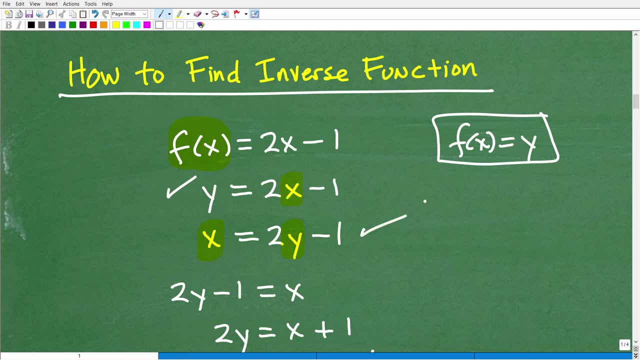 the y and the x right there. Okay, now, at this point, what you're going to do is you're going to solve for y. Okay, when you do that, you will actually will have found the inverse function. So let's go ahead and finish this. 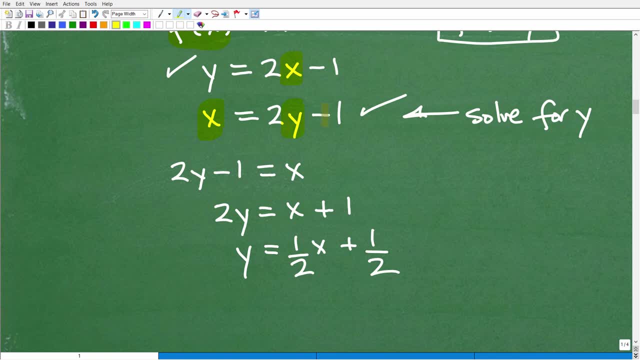 So we have: x is equal to 2y minus 1.. So the left is equal to the right, the right is equal to the left. So I'm going to put this: 2y minus 1 is equal to x. This is perfectly fine to do this. 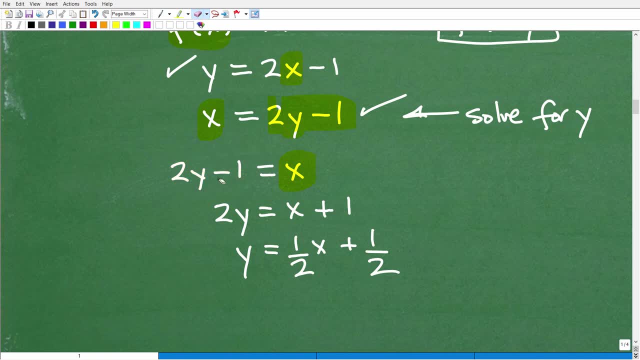 The reason why I'm doing that is because I like to solve for my variable on the left-hand side of the equation. So let's go ahead and solve for y. So my first step will be: I'm going to add 1 to both sides of the equation- and with 2y is equal to x plus 1- and then I'm going to divide everything. 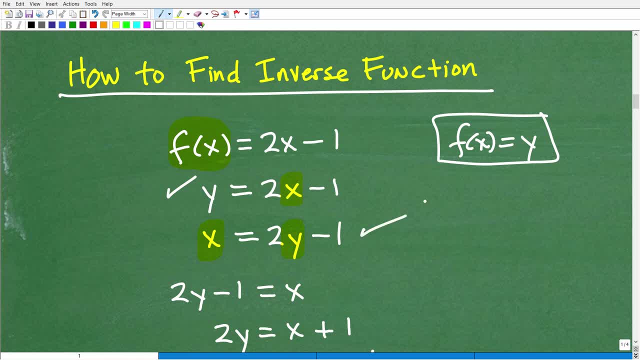 going to flip-flop the y and the x right there. okay, now, at this point, what you're going to do is you're going to solve y. okay, when you do that, you will actually will have found the inverse function. so let's go ahead and finish this particular problem. so we have: x is equal to 2y minus 1, so the left is equal to. 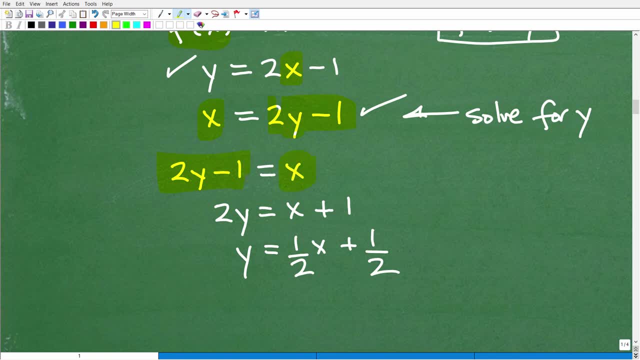 the right. the right is equal to the left, so I'm going to put this: 2y minus 1 is equal to x. this is perfectly fine to do this. the reason why I'm doing that is because I like to solve for my variable on the left hand side of the equation. so let's go ahead and solve for y. so my first step. 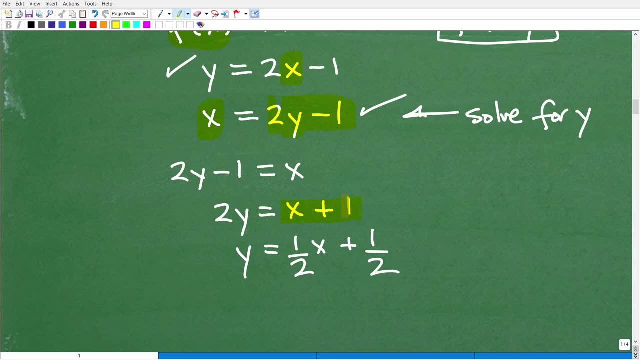 will be. I'm going to add 1 to both sides of the equation, end up with: 2y is equal to x plus 1, and then I'm going to divide everything by 2. okay, so here. your final answer could look like this: x plus. 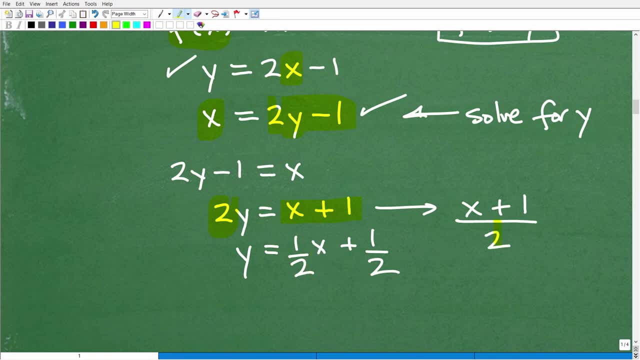 1 over 2, but I'm going to suggest that you write it this way: just put this to this denominator over this and over this, so you'll end up with one half x or x over 2 plus one half. okay, so this is equivalent to this, and there you go, okay. 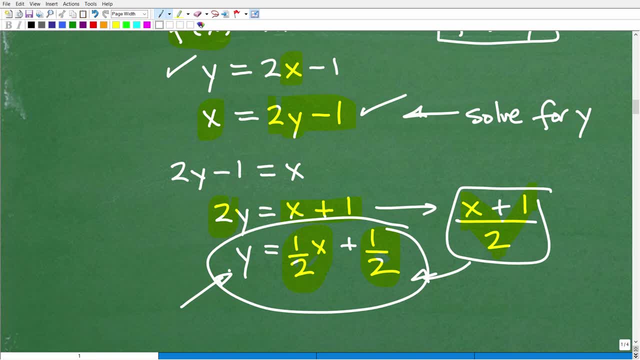 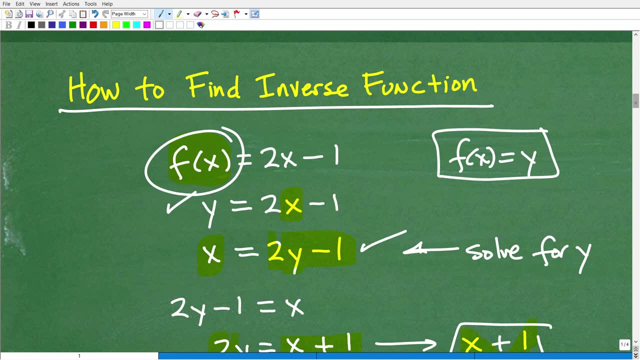 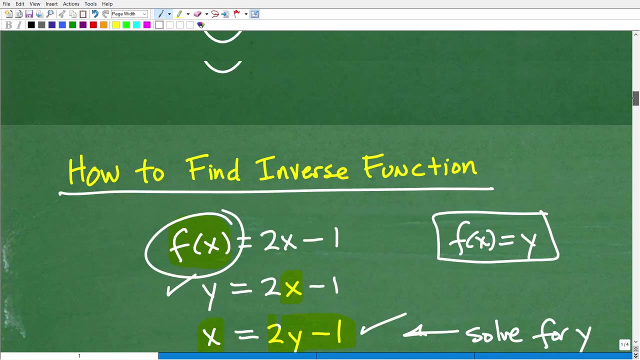 this right here is in fact the inverse function and uh, because we uh solved, okay, or because we had the function f f of x and it's inverse, right down here you're going to use this notation, this f negative 1 of x. okay, and this is basically the same functions. let me go way back up here. 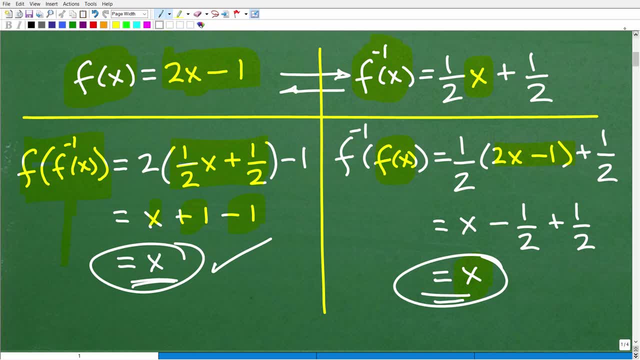 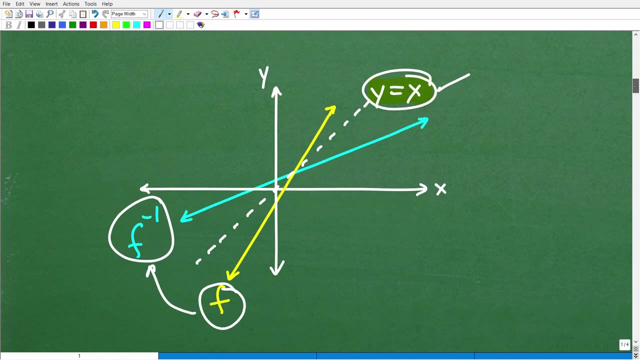 that, um, I was showing here with the composite right. so we just found that function inverse. it is this function, and when we plugged in the composite functions of one another, we both got x. that's how you can always check if, in fact, you have the correct uh inverse function. again, your teacher will require you. 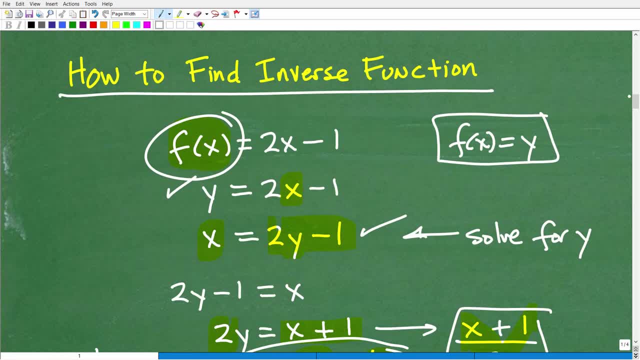 to do this if you have a good, you know strong- math teacher, someone that's really teaching you rigorous algebra. if you're not doing any of this, you're like, yeah, we don't do this in our class. well, guess what you're? you're, you're going to have gaps in your- in your- algebra education. you. 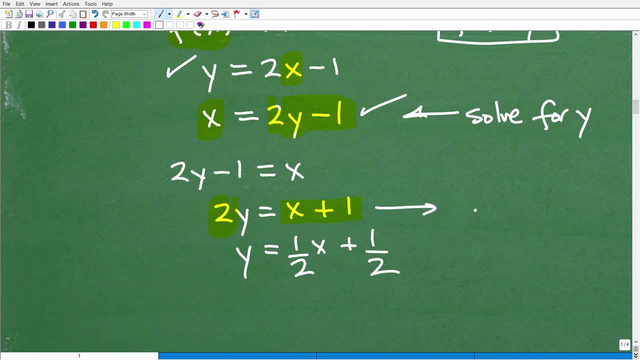 by 2.. Okay, So here your final answer could look like this: x plus 1 over 2,, but I'm going to suggest that you write it this way: Just put this to this denominator: over this and over this, So you'll. 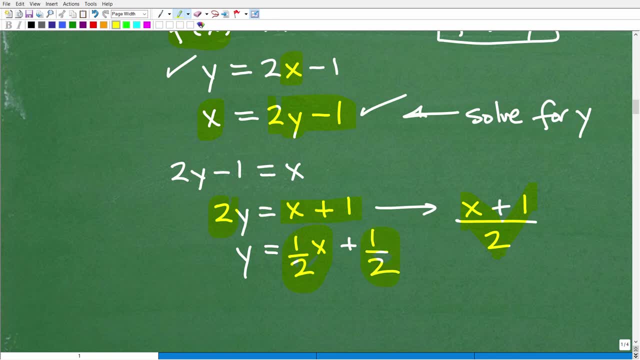 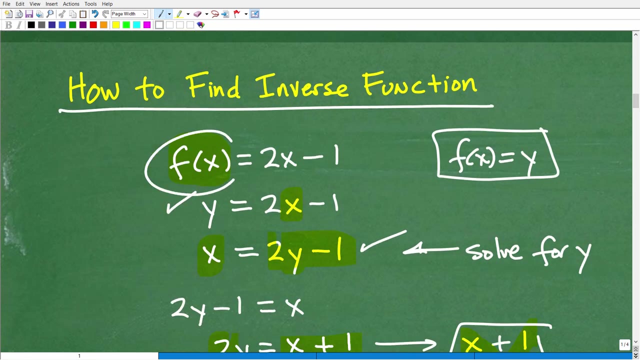 end up with 1 half x or x over 2 plus 1 half. Okay, so this is equivalent to this. and there you go. Okay, this right here is in fact the inverse function, and because we solved, okay, because we had the function f. 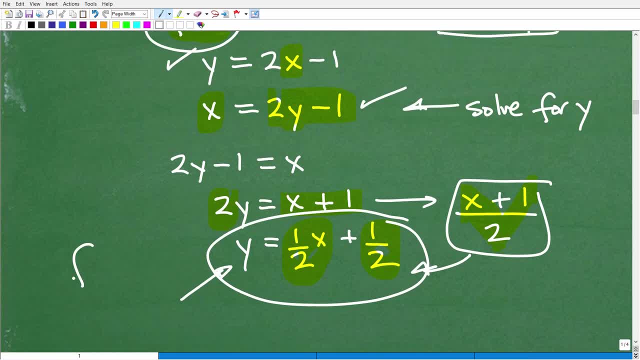 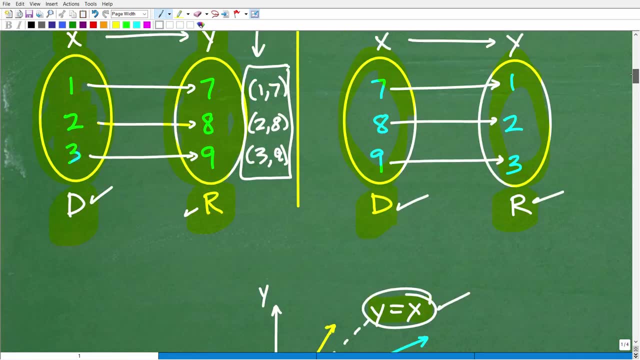 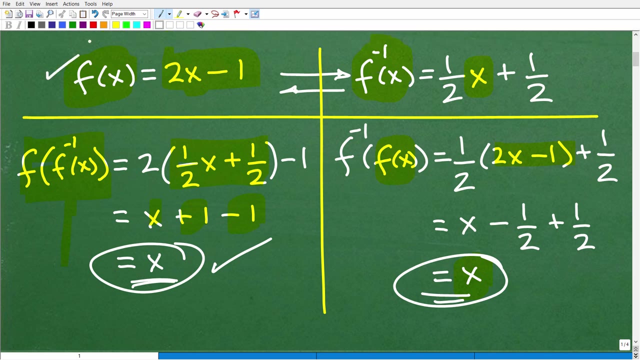 f of x and its inverse. right down here you're going to use this notation, this f negative 1 of x. Okay, and this is basically the same functions- Let me go way back up here- that I was showing here with the composite right. So we just found that function inverse. It is this: 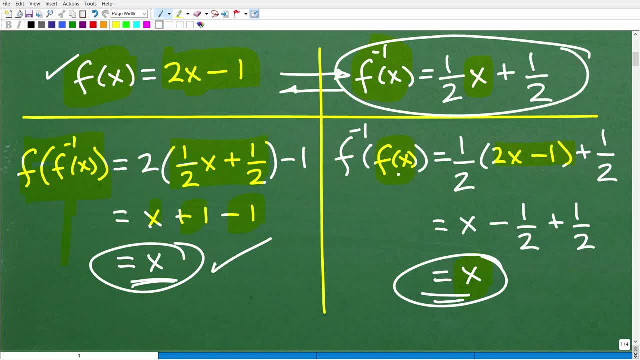 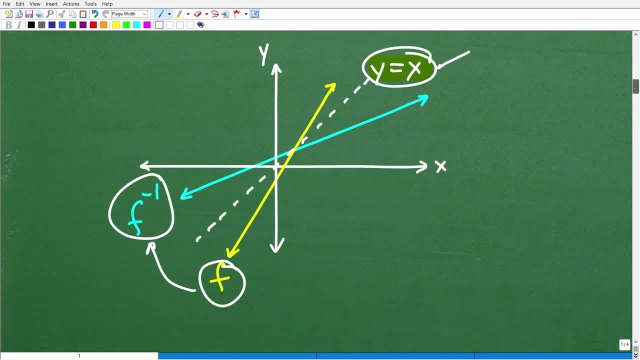 function, and when we plugged in the composite functions of one another, we both got x. That's how you can always check if, in fact, you have the correct inverse function. Again, your teacher will require you to do this if you have a good- you know strong- math teacher, someone that's. 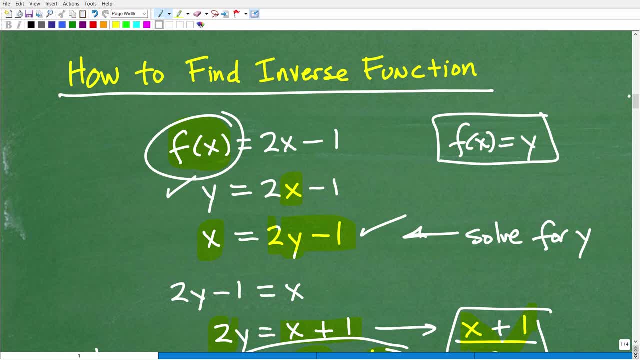 really teaching you rigorous algebra. If you're not doing any of this, you're like, yeah, we don't do this in our class. Well, guess what? You're going to have gaps in your algebra education. You might want to check out my full course so you don't miss anything important. Okay, so let's talk. 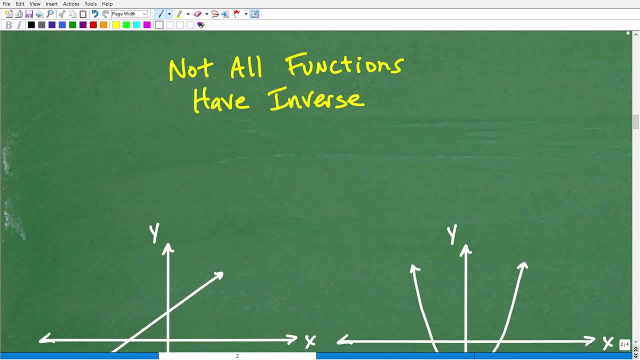 about, finally, why some functions do not have an inverse. So here's the deal, right, When you're first starting learning about relations, okay, now, some relations are functions- Okay, this is a review of stuff that you should know- And some functions have an inverse- Not all functions. 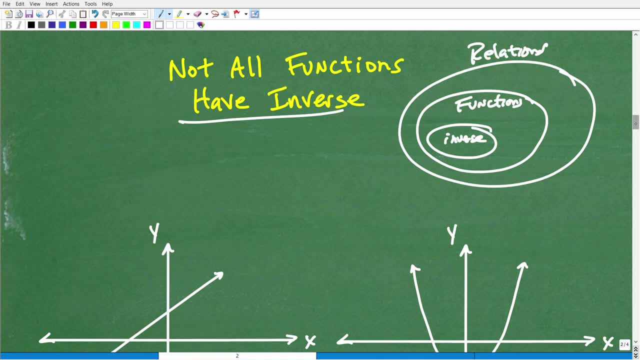 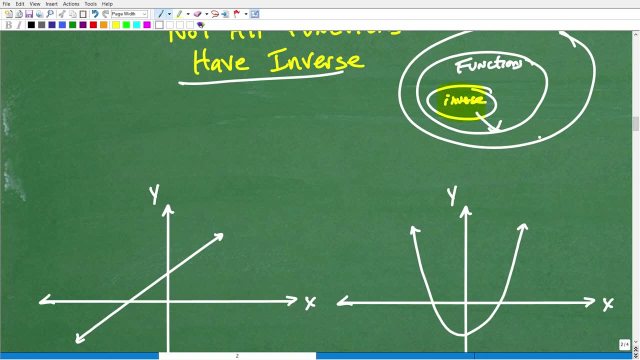 have an inverse. but how do we know that? Well, basically, the type of functions that have an inverse okay, or what we call one. I'll write it over here: one-two-one functions, one-two-one functions. So this is really, really important. So let's talk about some functions that have an 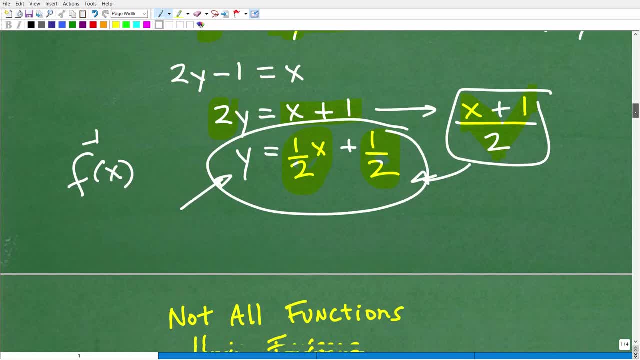 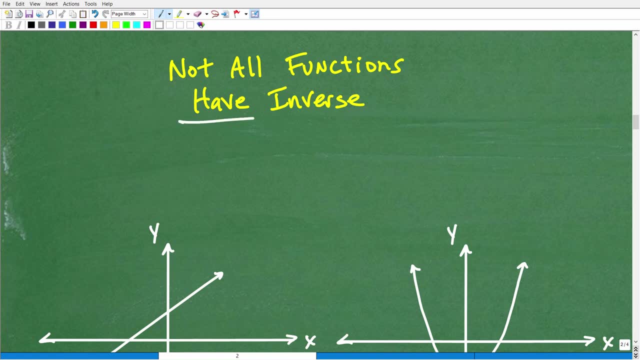 might want to check out my full course so you don't miss anything important, okay, so let's talk about finally, why some functions do not have in an inverse. so here's the deal. right, when you're talking about functions, remember you first start learning about relations. okay, now some relations. 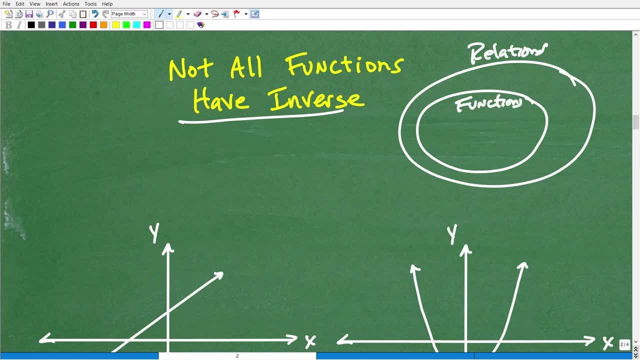 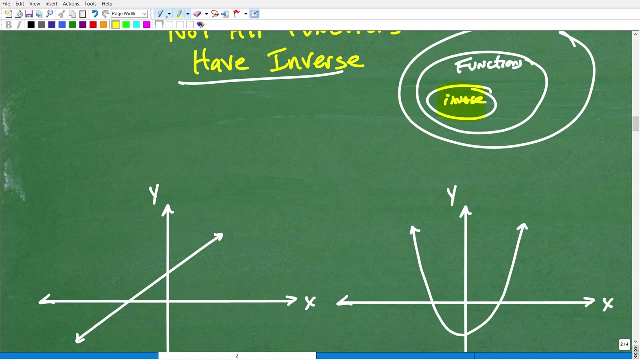 are functions. okay, this is a review of stuff that you should know, and some functions have an inverse. not all functions have an inverse, but, uh, how do we know that? well, basically, the type of functions that have an inverse, okay, or what we call one, i'll write it over here: one, two, one functions. one, two, one functions. so 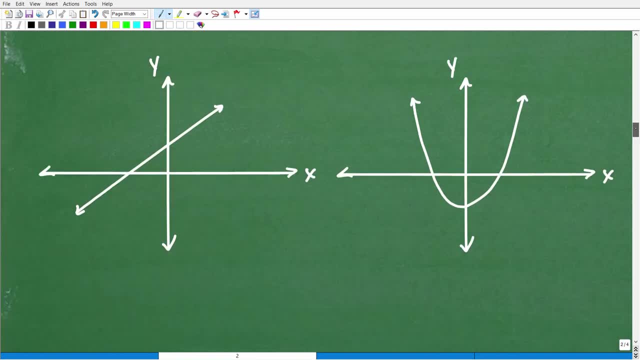 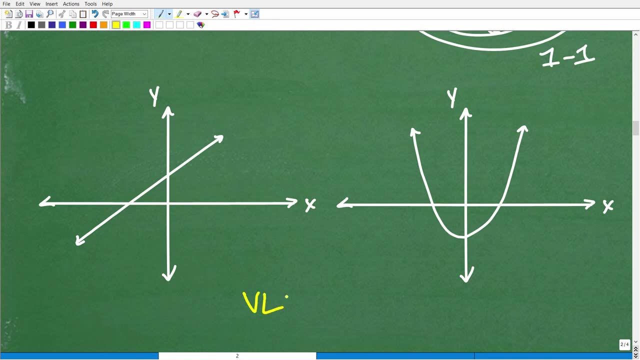 this is really, really important and let's go ahead and, uh, learn about one two. one functions. now, what you're going to need to understand here is to test the vlt and the hlt. okay, and that's not to be confused with the blt, which is bacon, lettuce and tomato, tomatoes, and see, i'll write. 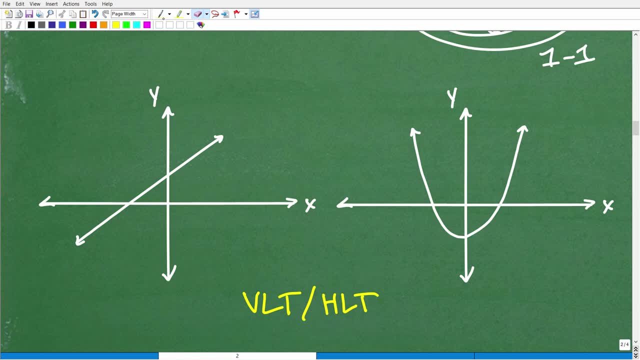 this stuff down, i get hungry anyways. vlt and hlt. so let's just quickly review the vlt. okay, this is the vertical line test. this is the test to determine whether a graph represents a function. so how does that work? well, if i draw a vertical line anywhere through a graph and it only chops through that graph one time, okay, like right. 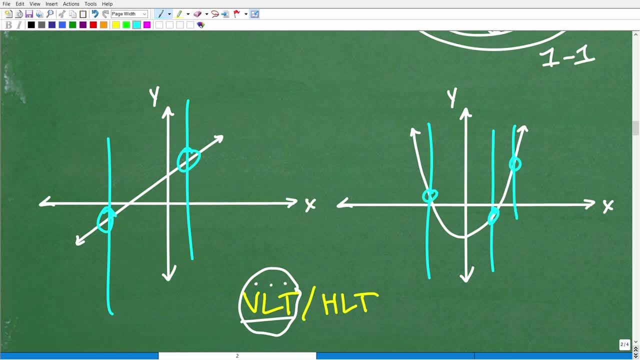 here, anywhere along this graph, it only intersects that graph once. well, that indicates that, uh, you are dealing with a function, okay. so in both of these examples, you're going to have a function right here. let me just erase this. uh, these graphs, um, are functions okay because they pass the vlt. 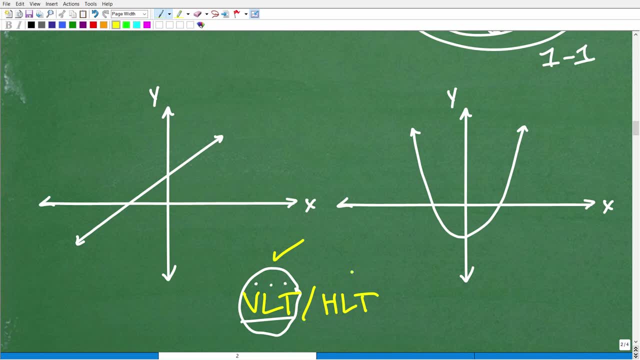 all right, so this is a graphical test that you want to know. so now let's talk about the hlt. what is the hlt? so this is called the vertical line test, right? i just drew vertical lines. so you might be saying, well, hlt, is that the horizontal line test? yes, indeed, and this is the test to see. 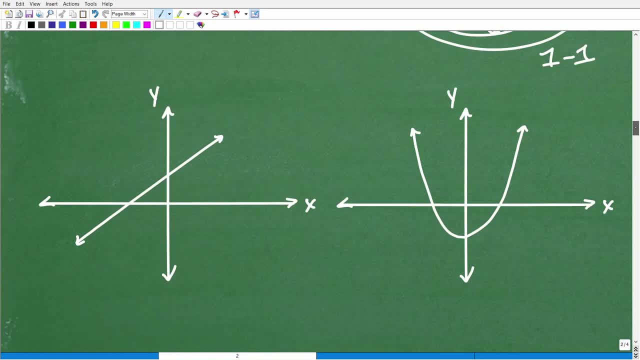 inverse. Okay, so let's go ahead and learn about one-two-one functions. Now. what you're going to need to understand here is two tests: the VLT and the HLT. Okay, and that's not to be confused with the BLT, which is bacon, lettuce and tomato, tomatoes, And see, I'll write this stuff down. 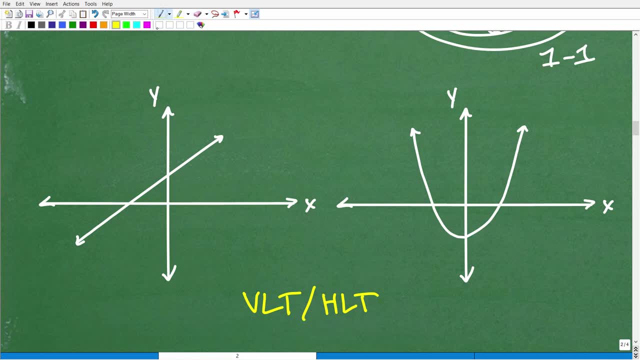 I get hungry. Anyways, VLT and HLT. So let's just quickly review the VLT. Okay, this is the vertical line test. This is the test to determine whether a glider is a vertical line test or a vertical line test. And this is the test to determine. 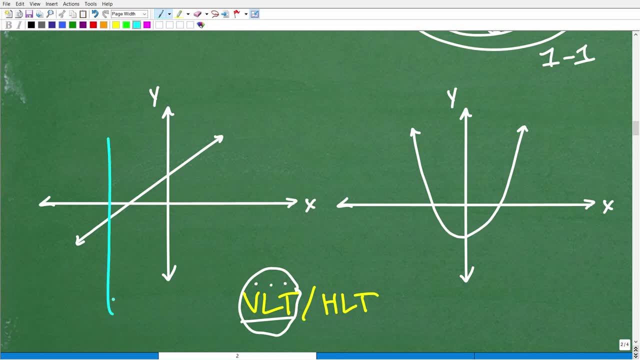 whether a glider is a vertical line test or a vertical line test, And this is the test to determine whether a graph represents a function. So how does that work? Well, if I draw a vertical line anywhere through a graph and it only chops through that graph one time, okay, like right. 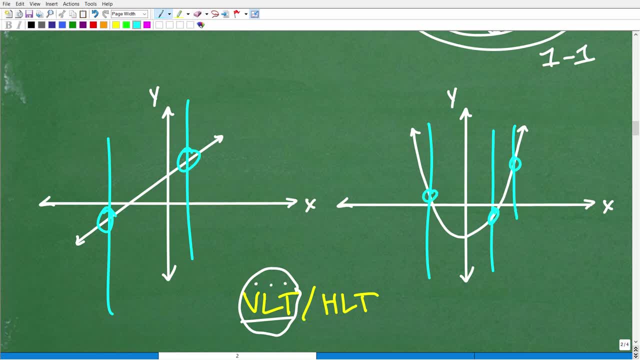 here, anywhere along this graph, it only intersects that graph once. Well, that indicates that you are dealing with a function Okay. so in both of these examples right here- let me just erase this- These graphs are functions okay because they pass the VLT. 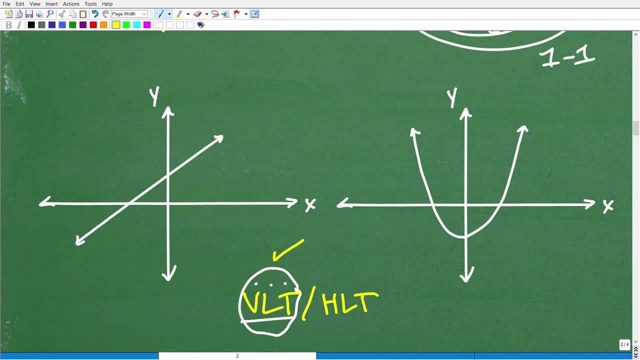 All right, so this is a graphical test that you want to know. So now let's talk about the HLT. What is the HLT? So this is called the vertical line test, right, I just drew vertical lines, So you might be. 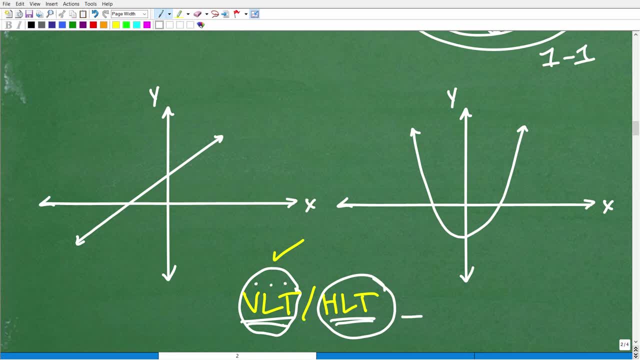 saying: well, HLT, is that the horizontal line test? Yes, indeed, And this is the test to see if you have a one-to-one function. All right, now let's go ahead and see how this works. So it works. 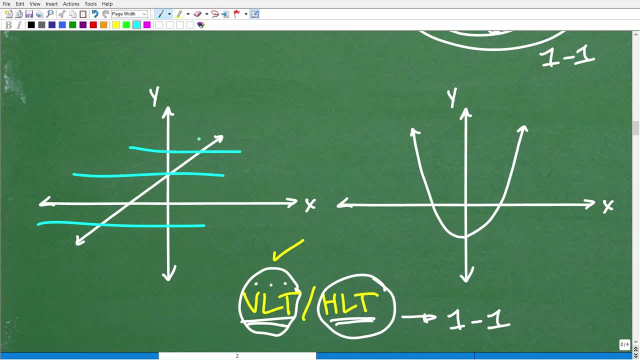 exactly like the vertical line test. You just draw a horizontal line through the graph. It just only chops through one time It passes. So this graph right here, this line, is a one-to-one function, meaning that it has an inverse, All right. so this right here could be like that: y equals 2x plus 1.. 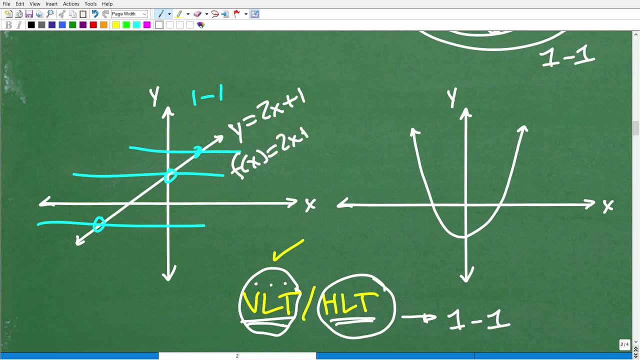 Of course I could write this as a function: f of x is equal to 2x plus 1.. I can't find the inverse, And, a matter of fact, we kind of just did that in those previous problem. Now let's take a. 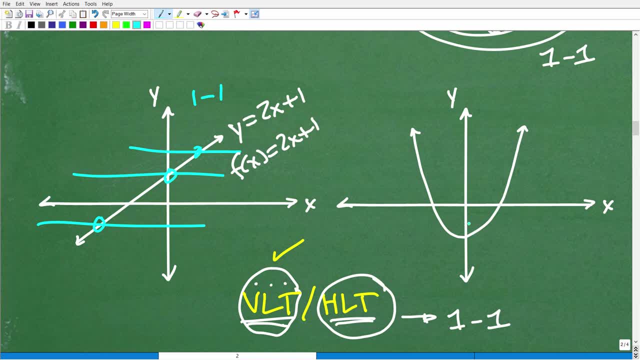 look at this situation. So this, again, is a function. It passed the vertical line test. But what's going on here? Well, the horizontal line is chopping through the graph two times. So if you have a graph and you draw a horizontal line and it can intersect more than once, it fails. 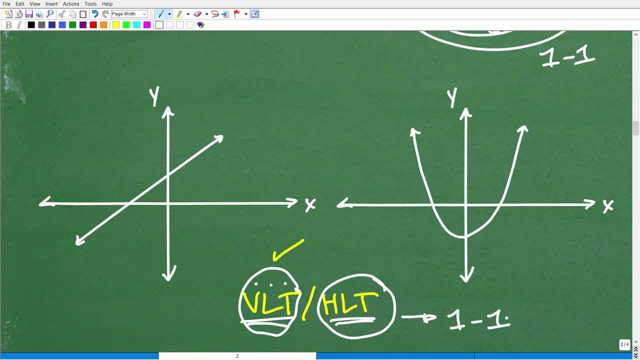 if you have a one-to-one function, all right. now let's go ahead and see how this works. so, uh, it works exactly like the vertical line test. you just draw a horizontal line, uh, through the graph. it just only chops through one time. uh, it passes. so this graph right here. this line is a one-to-one function, meaning that it has an inverse. all right. 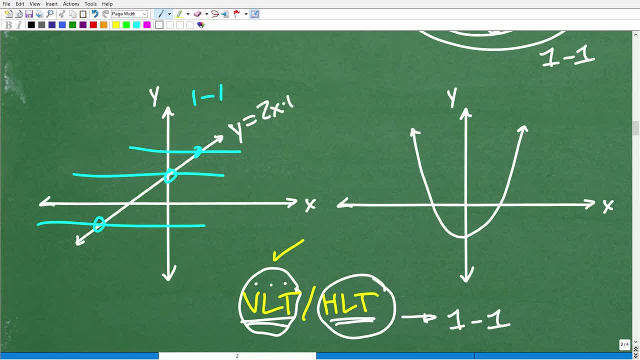 so this right here could be like that: y equals two x plus one. um, of course i could write this as a function: f of x is equal to two x plus one. i can't find the inverse, and, a matter of fact, we kind of just did that in those previous problem. now let's take a look at this uh situation. so 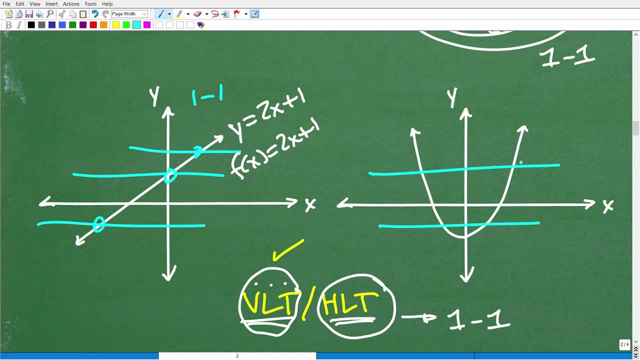 this, again, is a function. it passed the vertical line test. but what's going on here? well, the horizontal line is chopping through the graph- uh, two times. so if you have a graph and you draw a horizontal line and it can intersect more than once, it fails the hlt, meaning this is not a 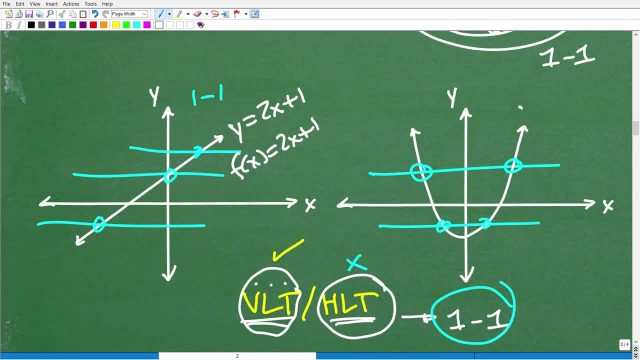 one-to-one function, meaning that you cannot find an inverse. so if you have a horizontal line and you have a graph, let's, let's say like: y equals x squared, actually, let me, uh, write this as a a function: f of x, maybe something like x squared minus two. all right, if i was to give you this. 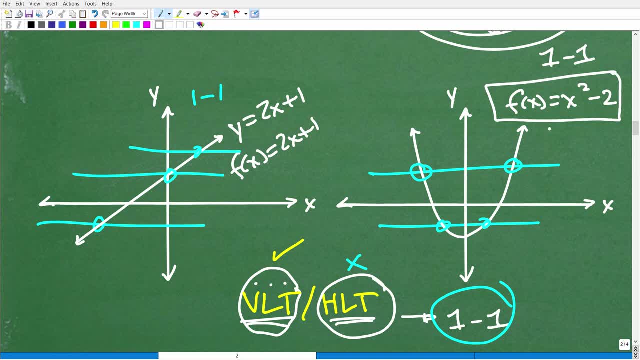 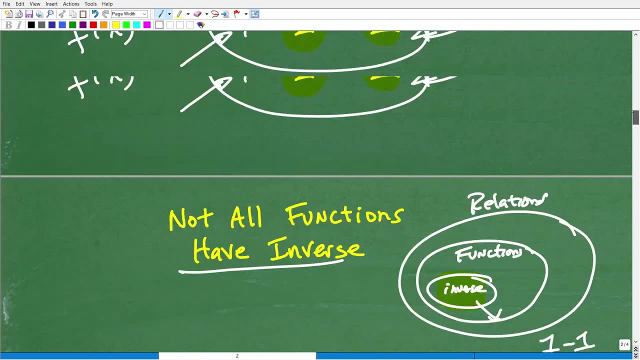 function. this is a function and you attempted to find the inverse function. you will have a problem doing that, okay, all right, so there you go. i don't know if it's been 10 minutes. i don't really pay attention, you know. i just try to come up with these snappy titles, but here's the deal. what i 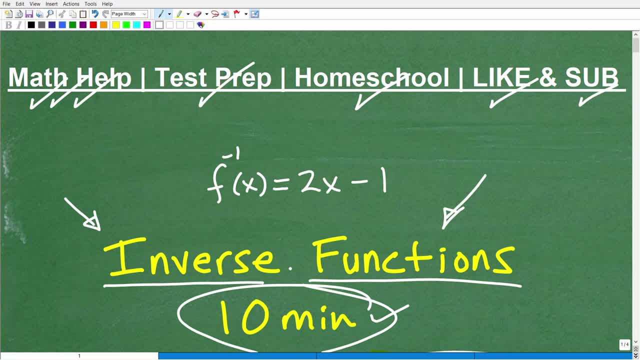 mean is that if you follow through and watch all my videos, you're going to definitely learn something about what i'm talking about, and hopefully we just upgraded your knowledge about inverse functions, again super important to know in algebra. and if you have, um, any more questions about functions, uh, please take advantage of all the videos on my youtube channel. i will have over 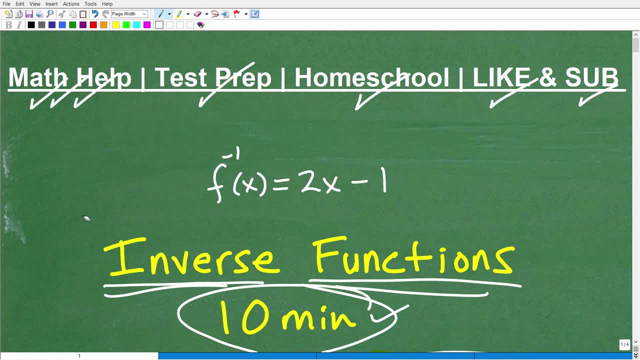 a thousand plus uh videos on my channel, ton of videos on functions, what they are, inverse function examples- but i really, really teach this heavy duty in my algebra courses. okay, all right. so, with that being said, i definitely wish you all the best in your mathematics adventures. thank you for your time and have a great day.